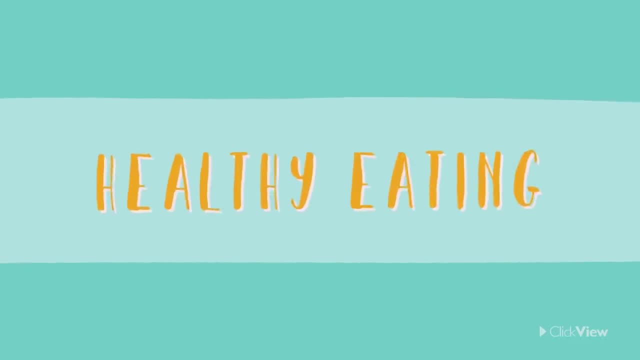 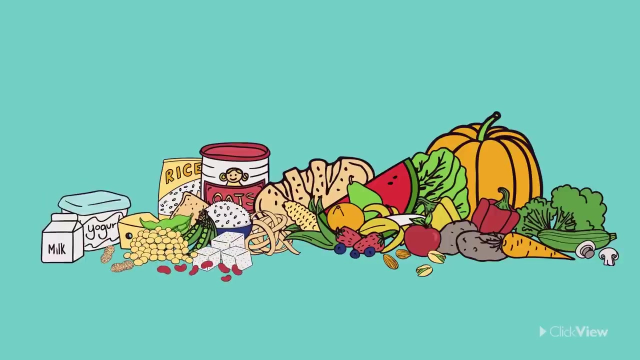 One of the most important healthy habits to have is healthy eating. Healthy eating is all about feeding your body fresh and nutritious foods. This should include colorful vegetables, fruits and nuts, grains, legumes, dairy and lean meats and fish. Even though all these foods are good for us, there are still some that we don't need to. 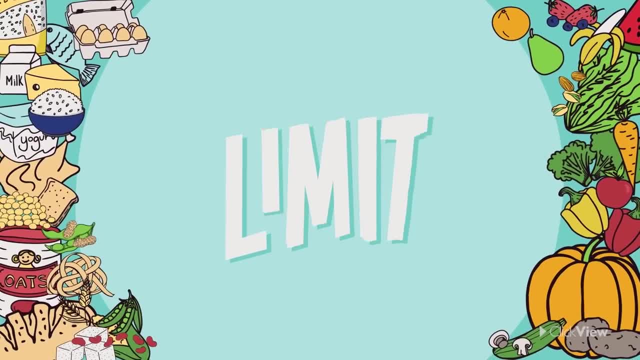 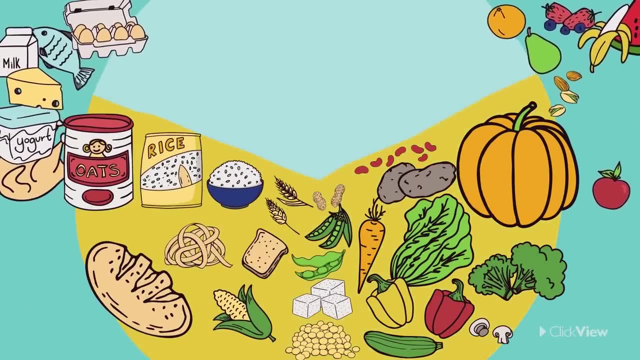 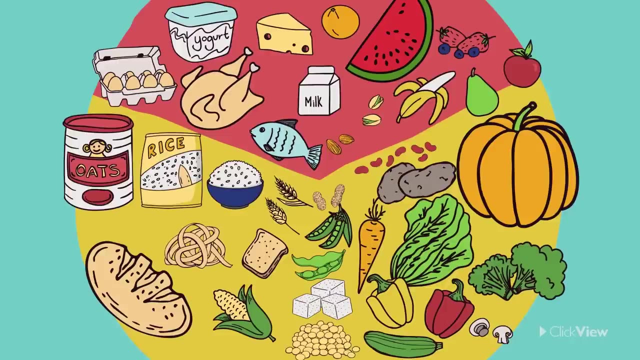 eat. There are some that we should eat lots of and some we should limit. We should eat lots of vegetables, legumes and grains, But we should eat lean meats, dairy and fruits and nuts in moderate amounts, which means not heaps and heaps. 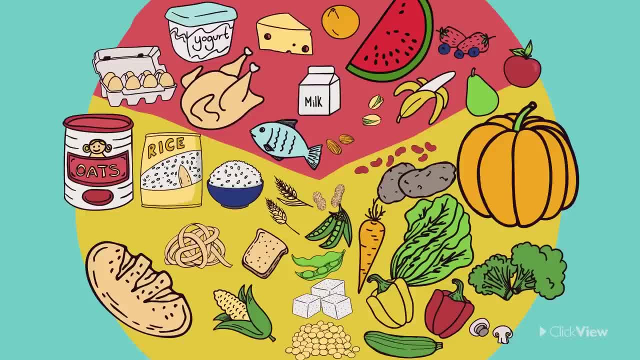 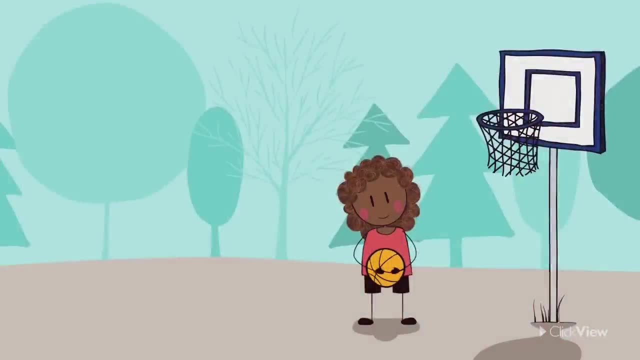 There are some foods that should only be a sometimes treat because they're not very good for us and have very little nutritional value, like sugary or fatty foods and drinks, And, of course, we should drink plenty of water every single day. When you combine healthy foods with physical activity, it will help you to feel healthy. 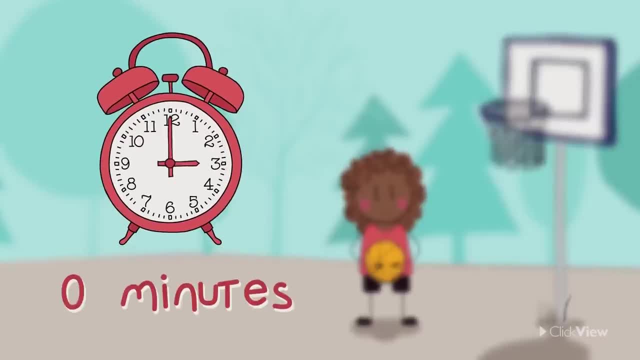 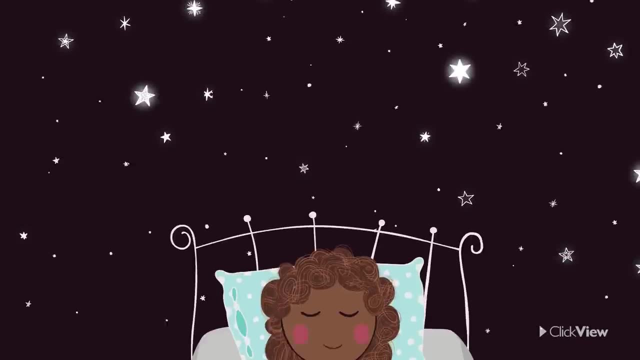 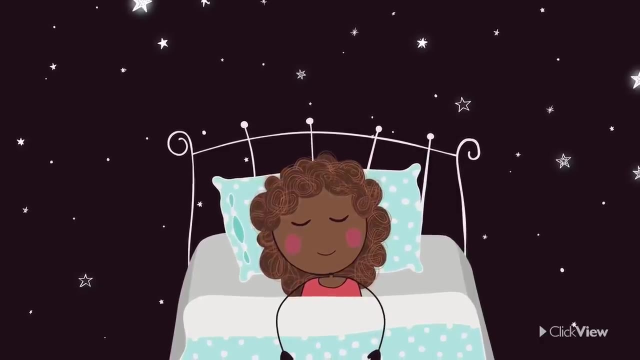 Did you know? children your age should be active for at least 60 minutes a day? Another healthy habit is getting lots of sleep. Sleep allows us to restore, repair and rebuild all of the things in our body, including our brain. Make sure you're getting 10 hours of sleep a night and you'll find yourself feeling 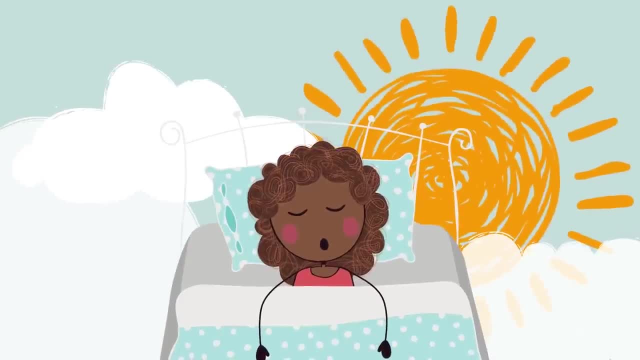 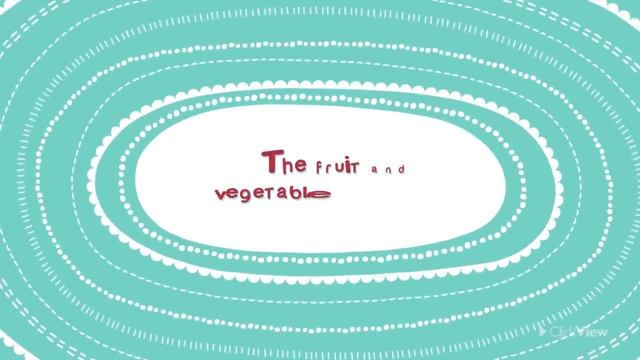 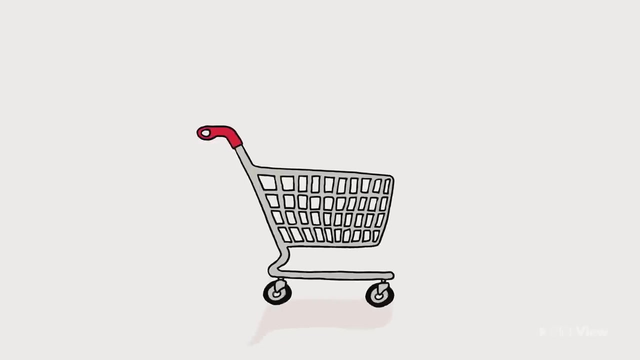 fresh and ready to make the most out of every day. Here are four ways you can build healthy habits. Eat the fruit and vegetable rainbow. Even though you may not be in charge of the grocery shopping, you can always make your own healthy choices. 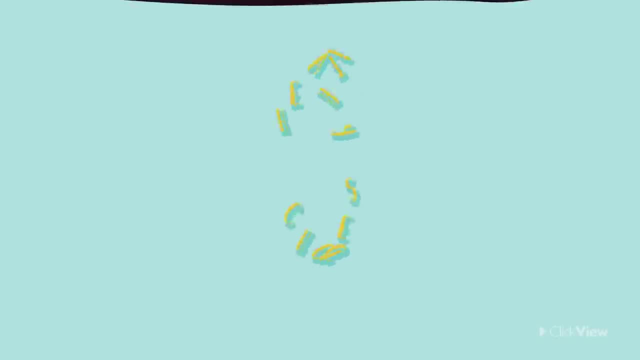 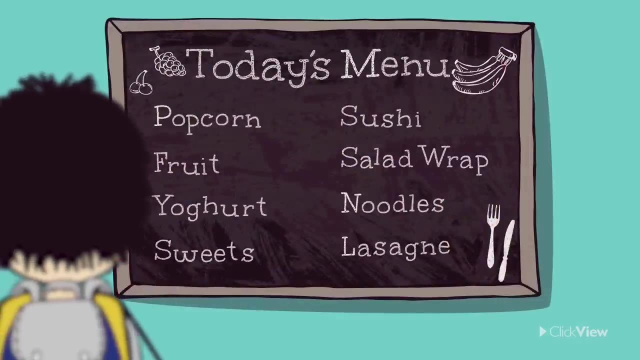 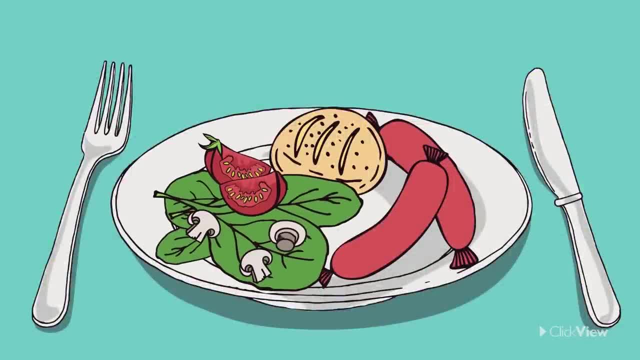 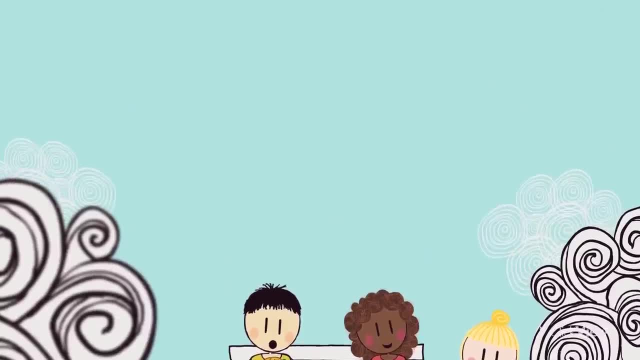 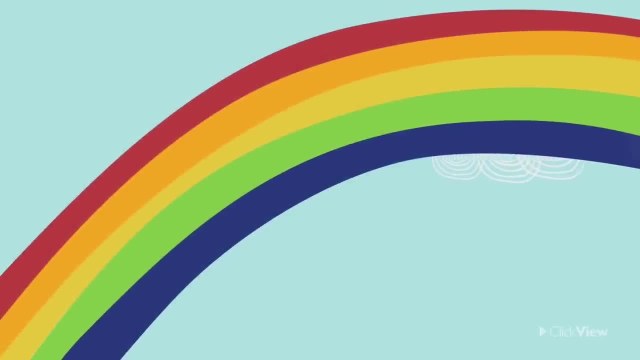 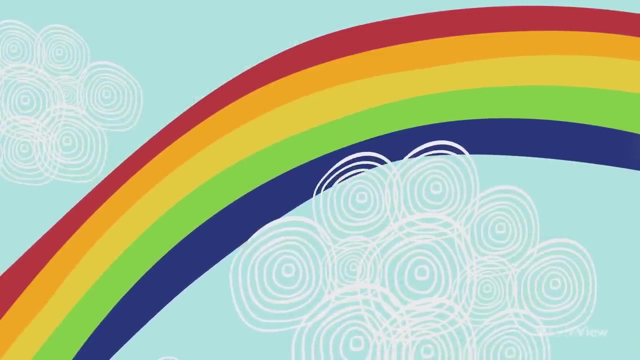 Or have some salad with dinner. Simple choices like that can make a huge difference to your health. Eating a variety of fruits and vegetables that are full of different colours is super important, because they help your body in different ways, So try and have as many colours as you can every day.